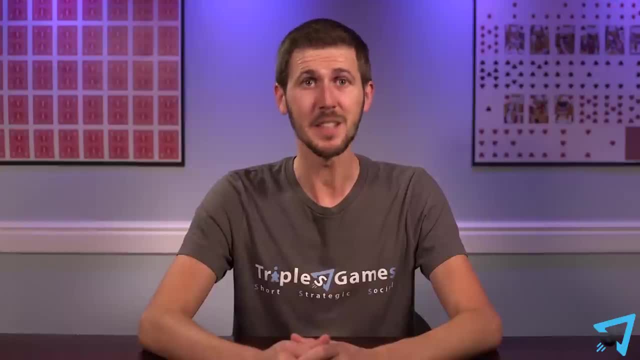 Scrabble how to play. The object of the game is to score the most points when the game ends. The game ends once one player has emptied their rack of all letters. when the bag is empty, or if all the players pass twice in successive turns, Lay out the board and give each player. 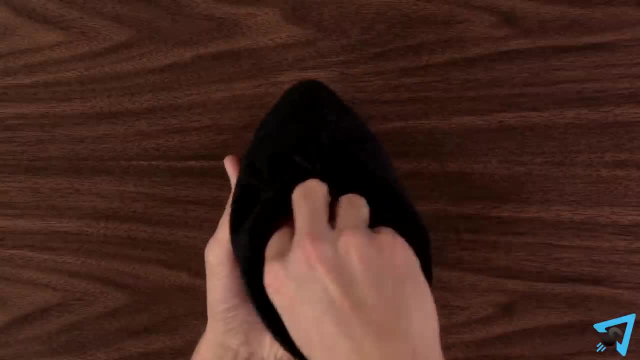 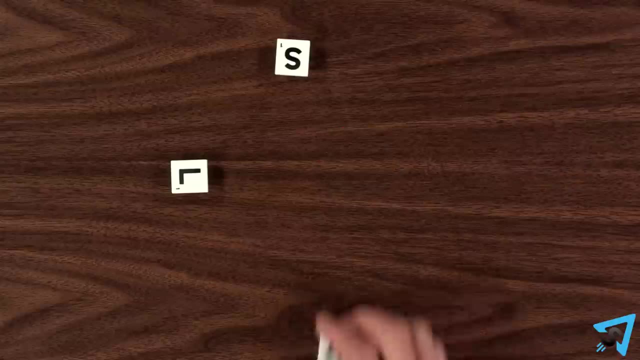 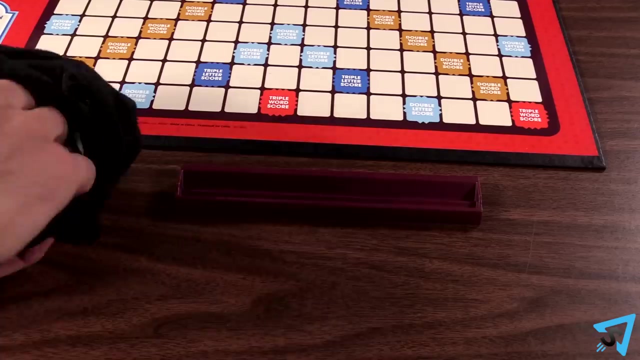 a tile rack. Mix up all the tiles in the bag and each player takes one tile. The player whose tile is closest to the letter A goes first. If it is a tie, try again. A blank tile beats any letter. Return the tiles to the bag, then, beginning with the starting player and proceeding clockwise. 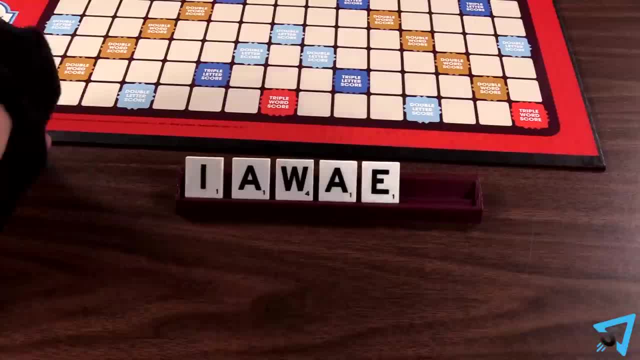 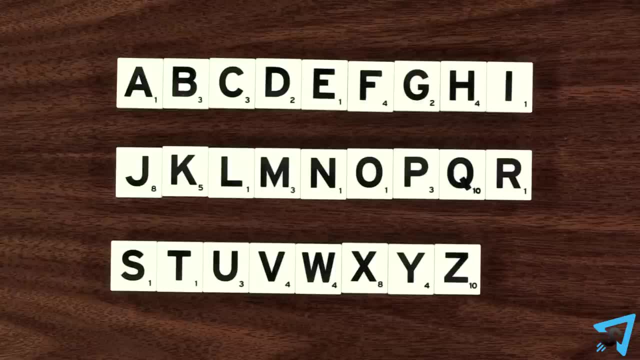 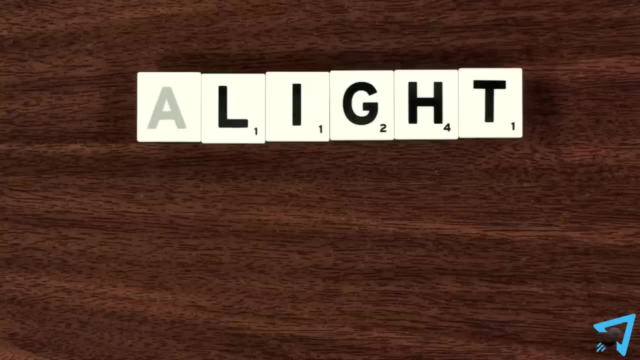 each player secretly draws seven random tiles and adds them to their rack. Tiles should remain hidden from your opponents. Each letter tile has a value as indicated by its number. Blank tiles have no value but can be used as any single letter. When played, you must declare its letter. 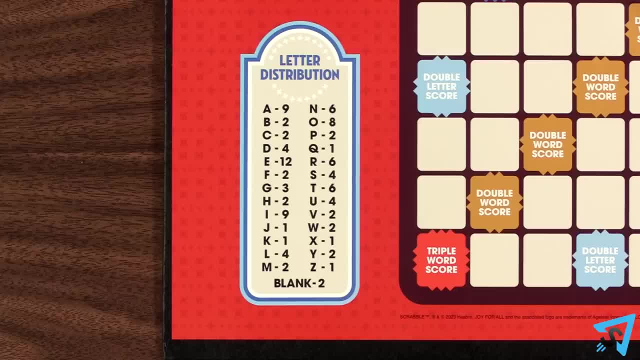 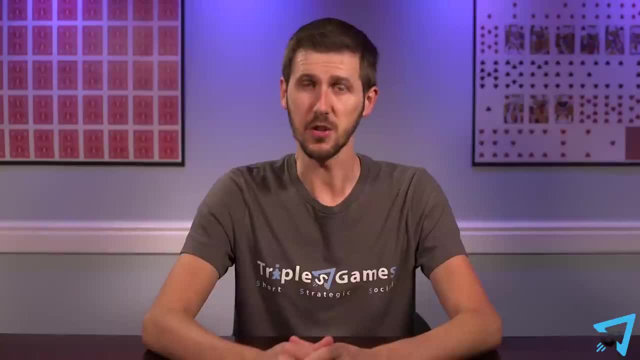 and you cannot change its letter later. The total quantity of each letter is printed on the board. After each player has their starting tiles, the game begins On your turn. you must form one new word on the board, or discard and draw new letters, or skip your turn. The very first word of the game. 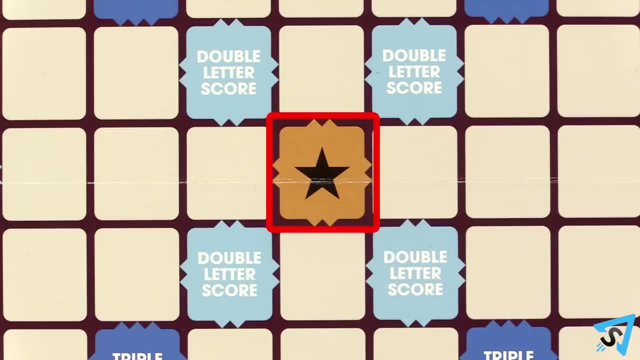 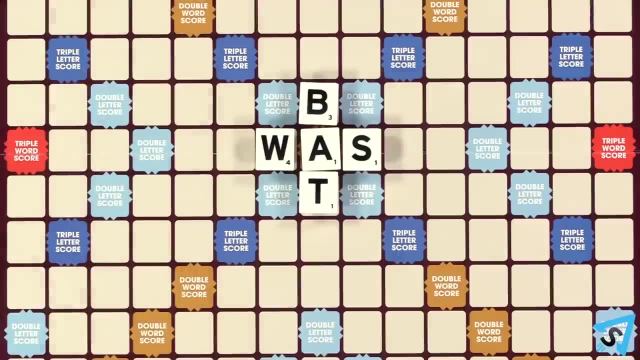 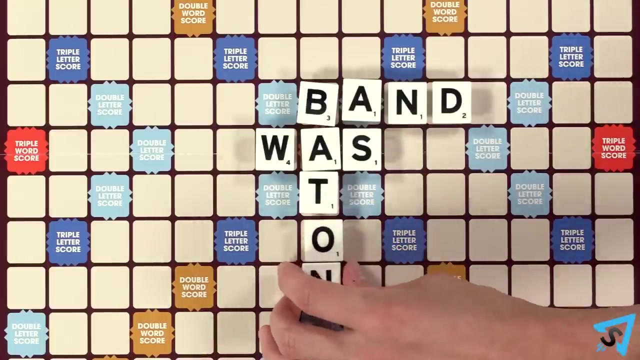 must be at least two letters long and cover the center. start square. After that you must form words on the board that are horizontally or vertically connected to a previously formed word. Words always read from left to right and top to bottom, Never backwards, upwards or diagonally. All placed letter tiles must be adjacent to each other. 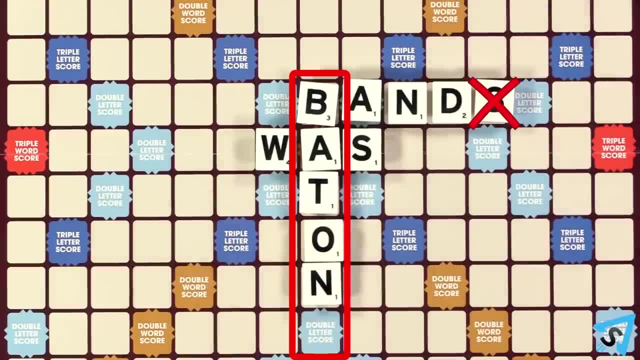 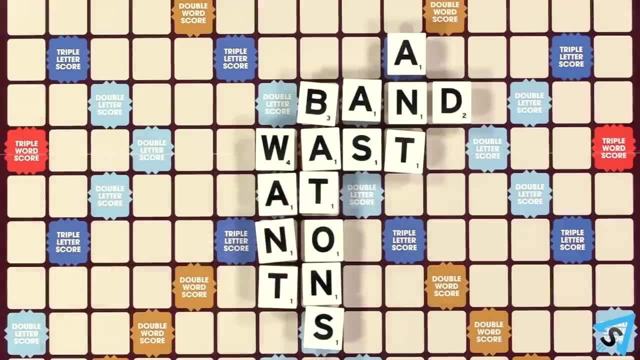 in a straight line and be a part of the same word. You cannot place letters in multiple locations across the board in a single turn. You are allowed to create multiple words by placing tiles adjacent to multiple words already in play. If you do, then all touching letters must form complete words. 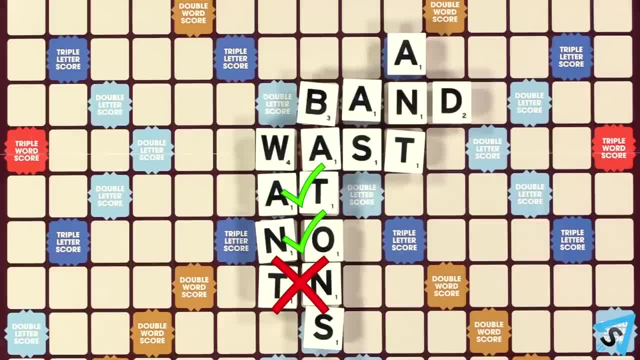 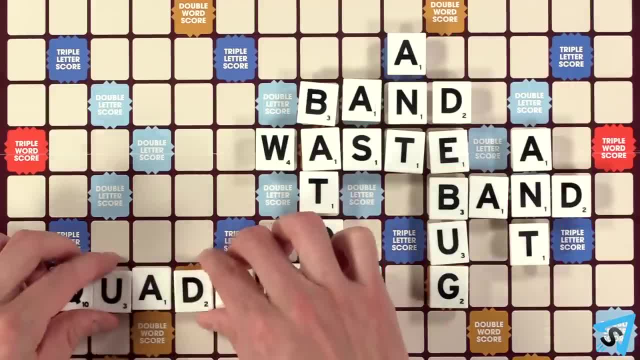 If even one word is not in play, the pattern will be changed and you will have to create a new. one is incomplete, but the rest are good. you may not play there. You may have any number of duplicate words on the board After you place your word. you then score points based on the combined value. 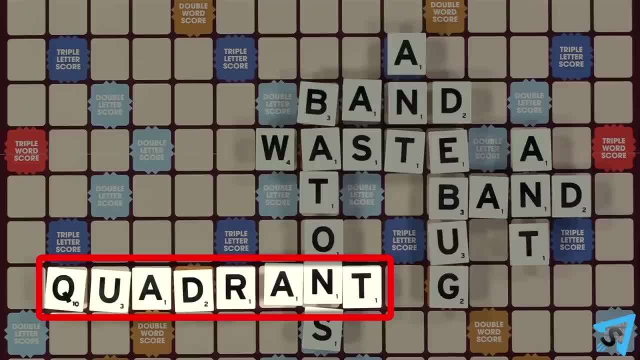 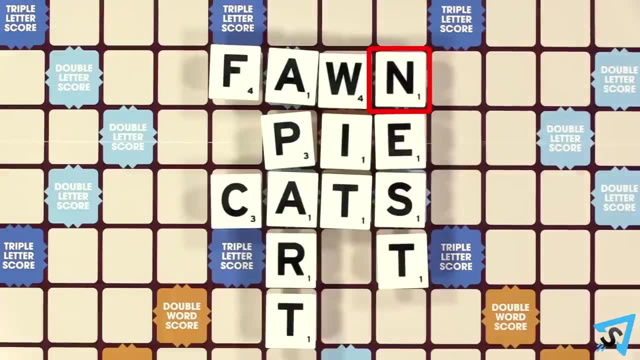 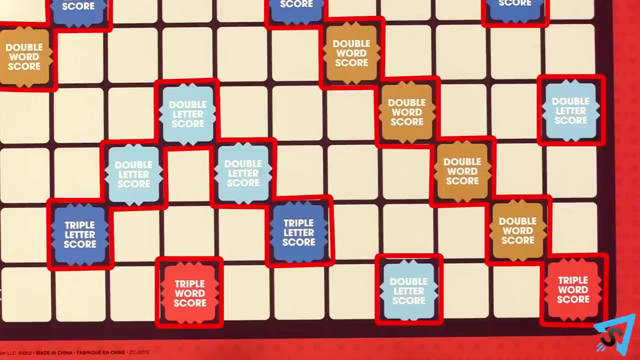 of all the letters in all the new words you formed that turn, At least one letter needs to be added to a word for it to be considered a new word. Letters that are a part of two different words will be scored twice once in each word. If you cover a premium square, then that word will score. 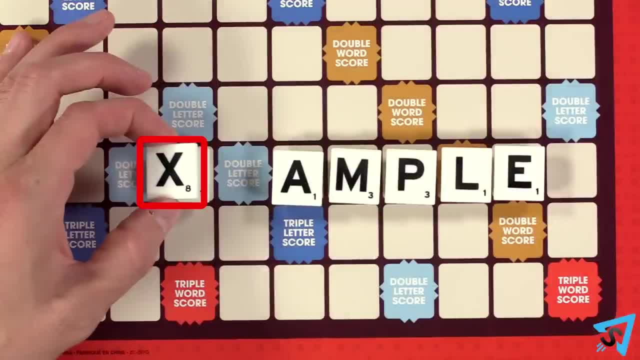 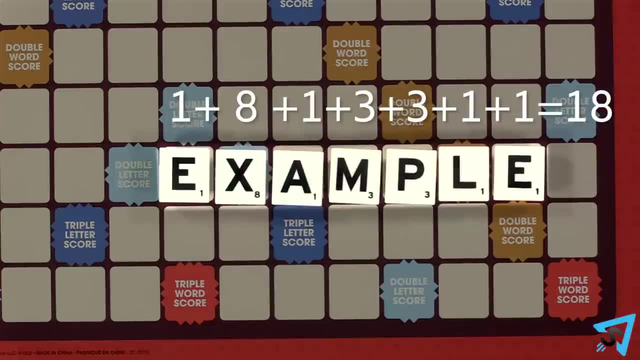 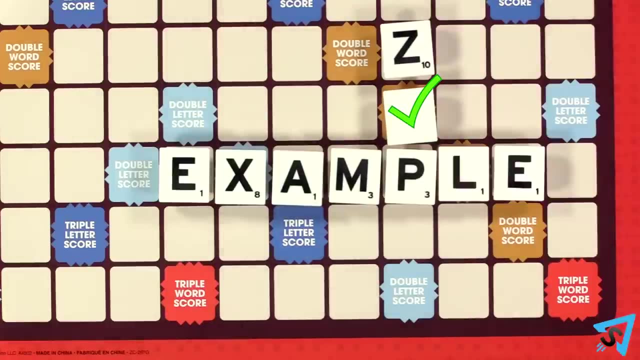 bonus points. The premium letter bonus only applies to the letter on top of it, while the premium word bonus applies to the total value of the word. Apply bonuses to premium letters first before applying premium word bonuses. Blanks on premium word squares still activate the bonus. You can only 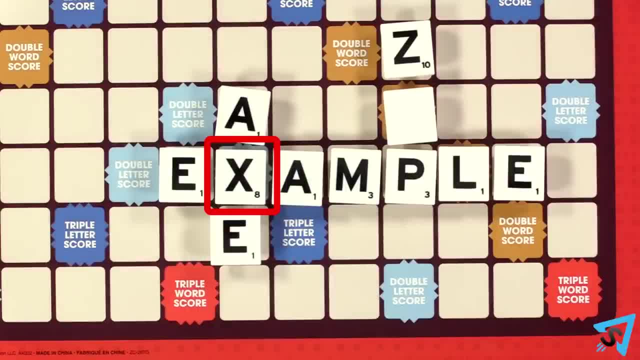 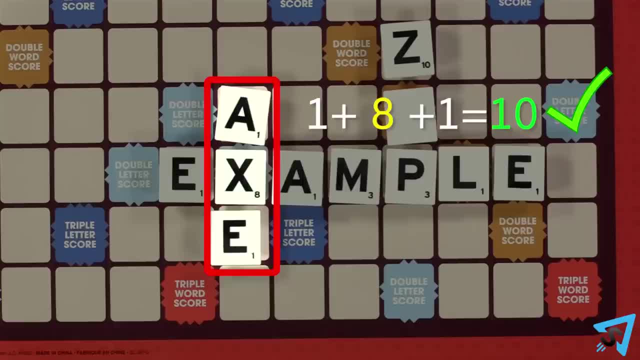 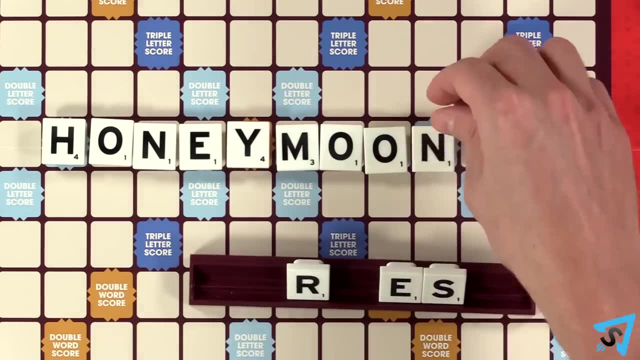 score premium bonuses. the turn you play Place the tile on the bonus. If you make a new word from an existing word that already had bonuses from a previous play, then you do not score those bonuses. The center start square is a double word bonus If you create a word using all seven letters on your rack in a 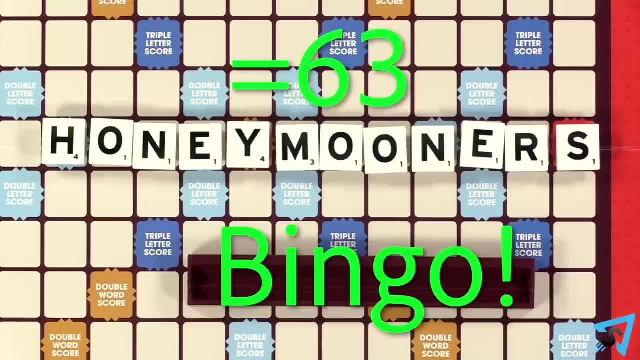 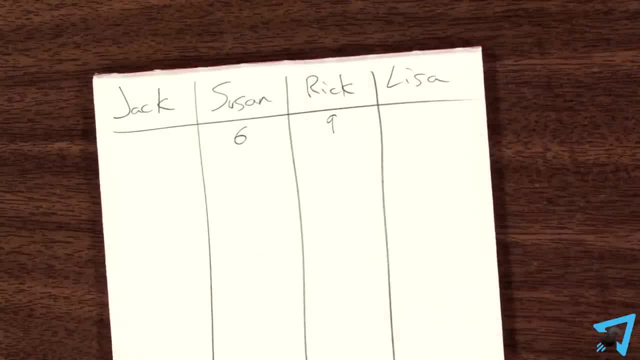 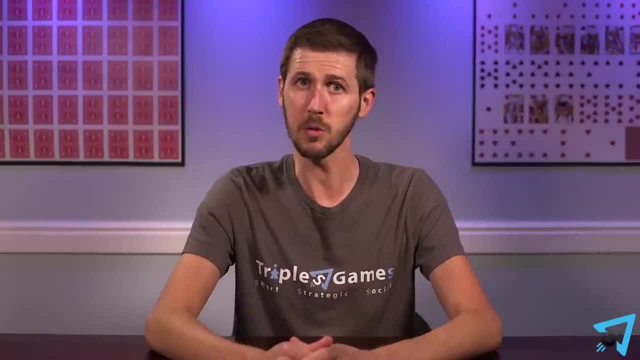 single turn, then that is called a bingo and you receive a bonus: 50 points after the word has scored. After you play your tiles, record your score on a scorepad, then draw back up to 7 tiles and the next player goes. You are allowed to use any word in an official Scrabble dictionary or 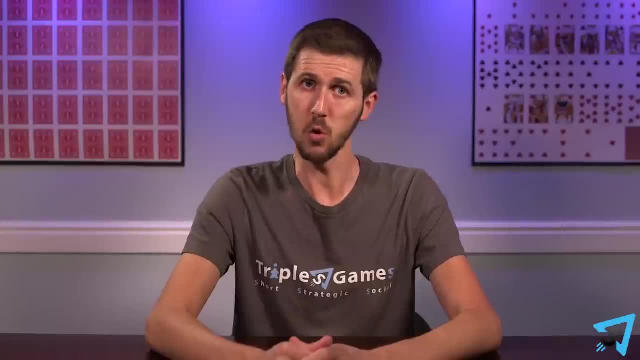 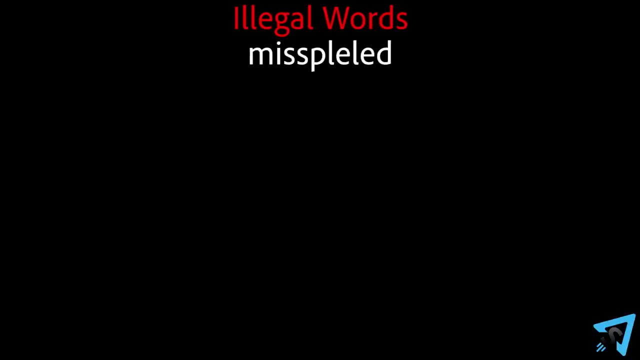 any agreed-upon dictionary of your choice. Players may only consult a dictionary during a challenge. Illegal words that are not allowed are any word that is misspelled, made-up words, proper nouns and proper names, foreign words, abbreviations, acronyms, freestanding prefixes and suffixes. 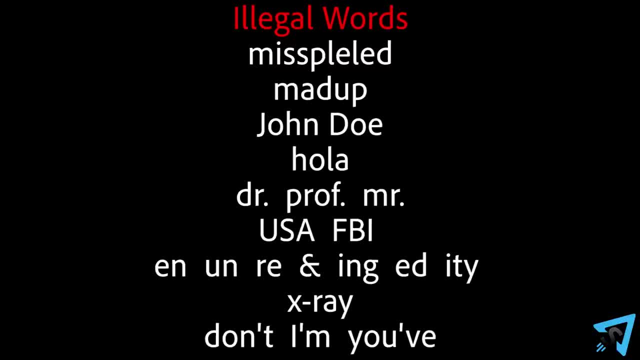 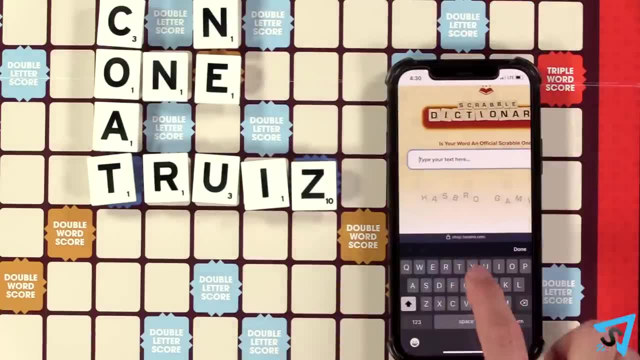 hyphenated words and words with apostrophes. If you think someone's word is illegal, you may challenge that word before the next player starts their turn, Look up the word in the dictionary. If the word is illegal, then the illegal word is returned to that player's ISRAC. 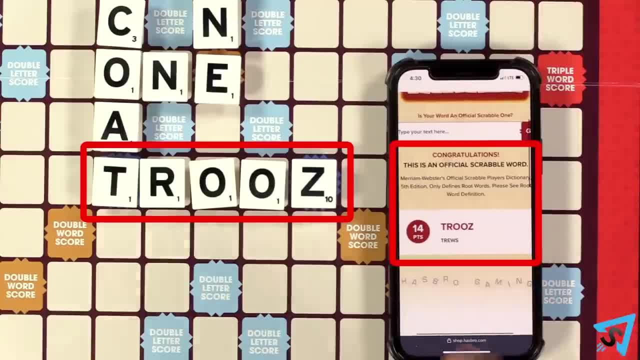 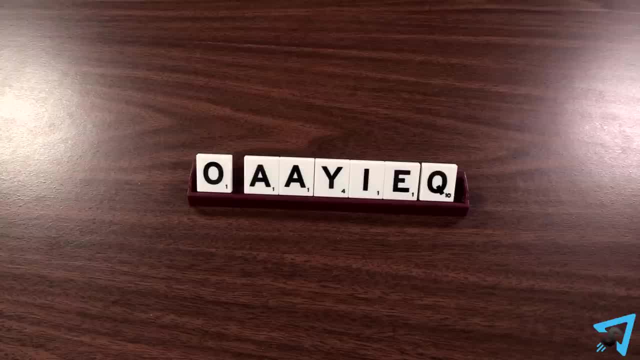 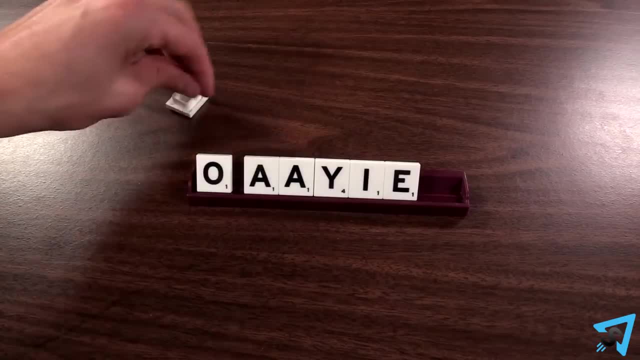 and no points are scored and their turn ends. If the word is legal, then the word remains and points are scored, but the challenger loses their next turn. If you are unable to play a word or choose not to, you may trade in tiles for new ones from the bag. Place all the tiles you wish to trade. 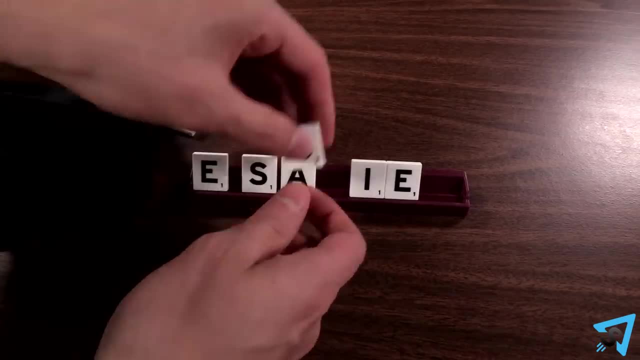 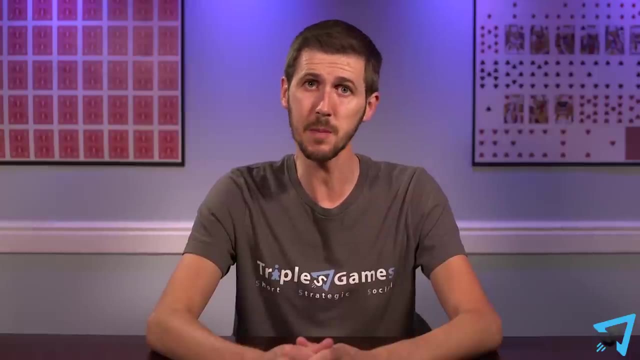 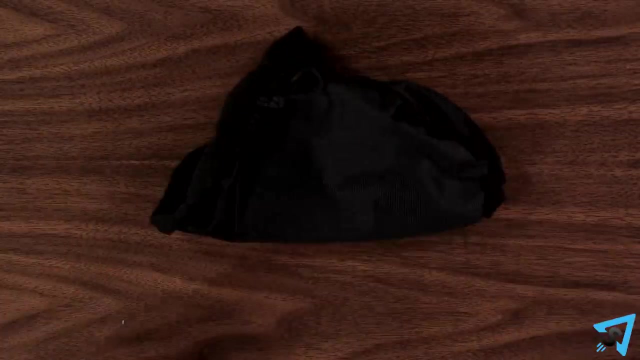 face down on the table, then draw the same number of tiles from the bag. Then return the face down tiles to the bag and end your turn. If you want, you may also choose to skip your turn without playing or discarding. Keep playing until the bag runs out of tiles. then play continues without players replenishing.